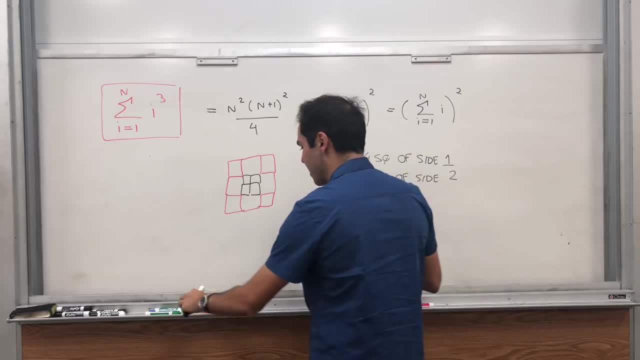 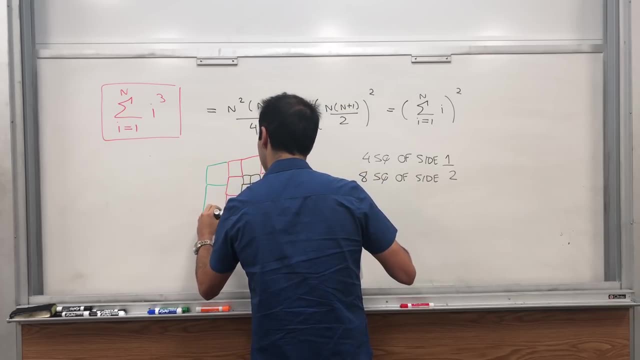 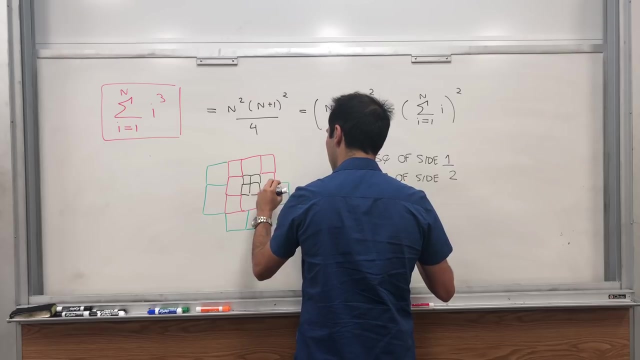 And then continue. do 12 squares of side three, which I believe looks something like that: One, two, three, four, five, six, seven, eight, nine, 10,, 11,, 12.. Look how pretty it is. 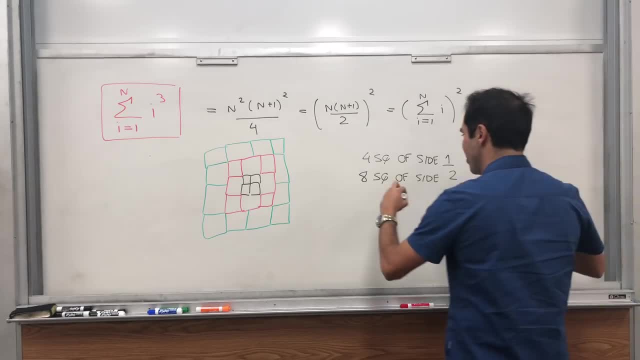 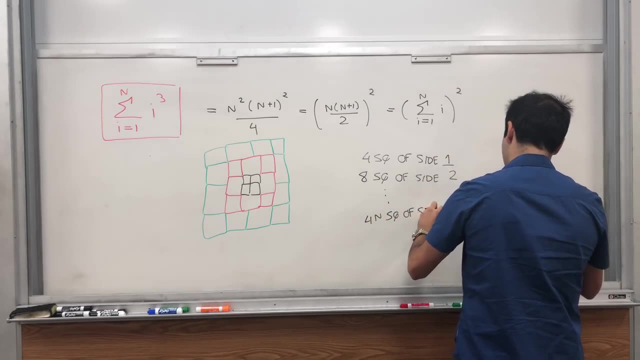 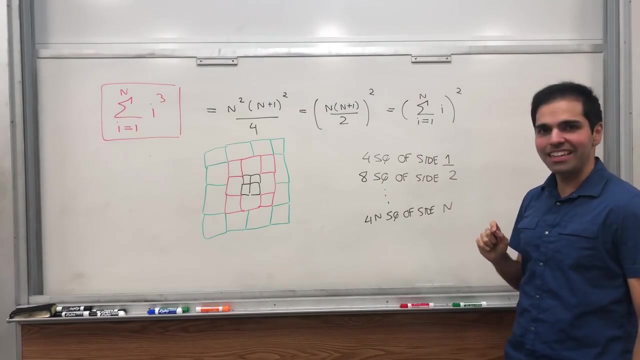 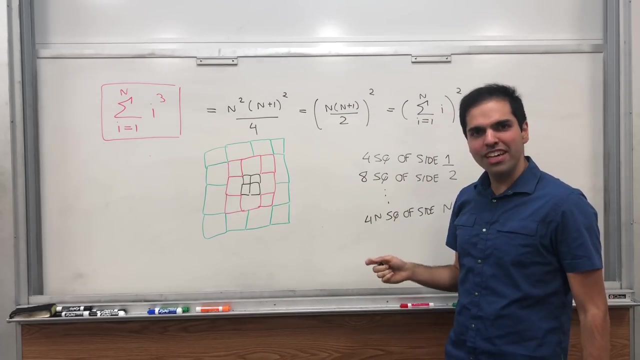 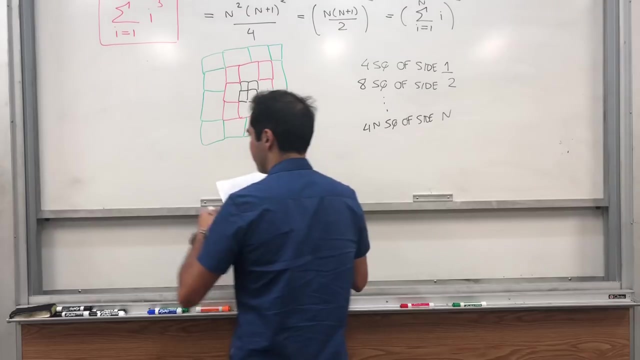 It's a nice flower, if you want. And in general, what you have is four n squares of side n, And calculating the sum of cubes and showing this identity actually just amounts to calculating the total area of this figure in two different ways. Because, on the one hand, what is the total area? 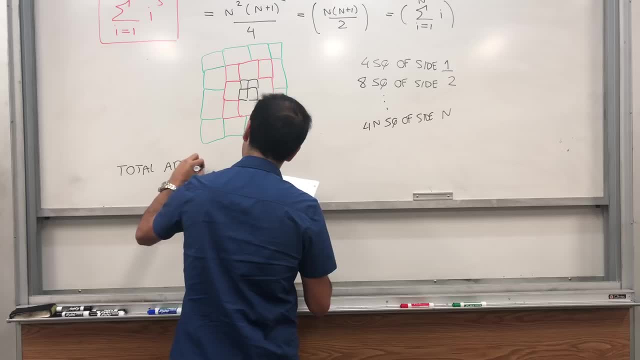 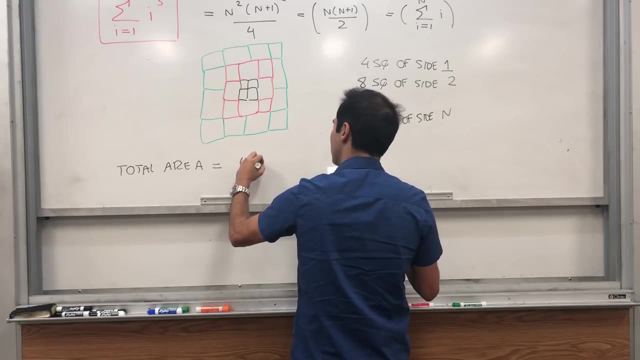 Four n squared, And on the other hand, what is the total area? All you do, you first sum up the squares of side one, and there are four of them, So four times one squared, And then you sum up the area of the red squares. 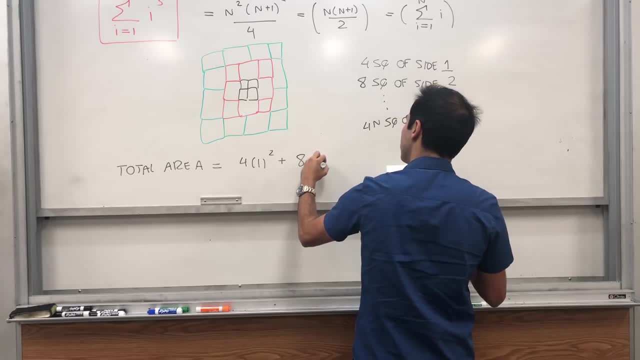 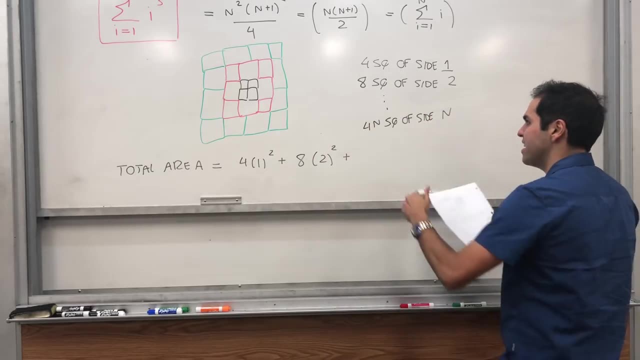 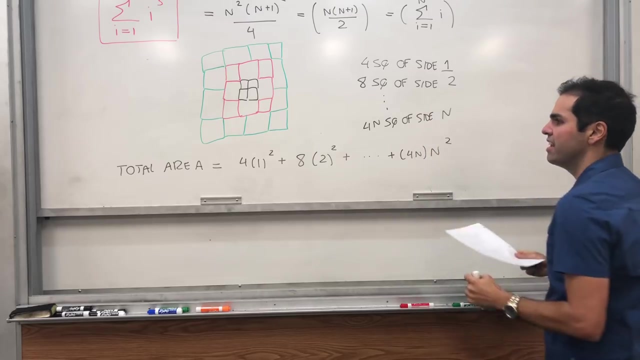 which is, remember, eight squares of side two, so eight times two squared. And then what is it? 12 times three squared, et cetera, et cetera, Until you get, yeah, 22 squared, 4n squares of sine n, whose area is n squared and it doesn't look like it's. 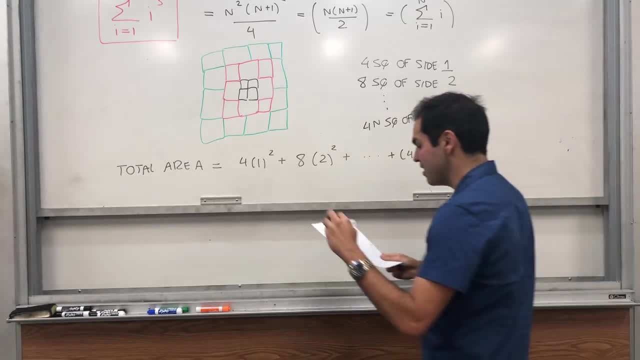 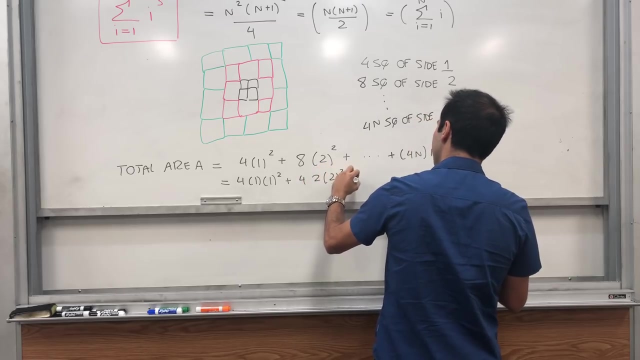 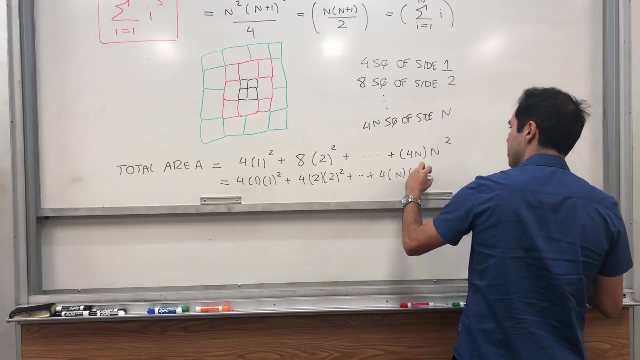 the sum of cubes. but let's manipulate this a little bit, because, notice, this is 4 times 1 times 1 squared. okay, why am I wasting my time with that? then 8. notice it's 4 times 2 times 2 squared, plus 4 times n times n squared, and this is 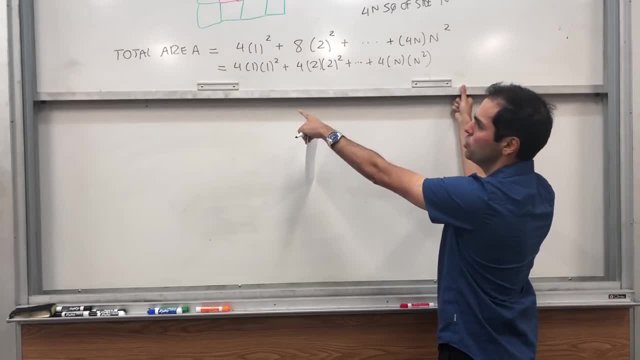 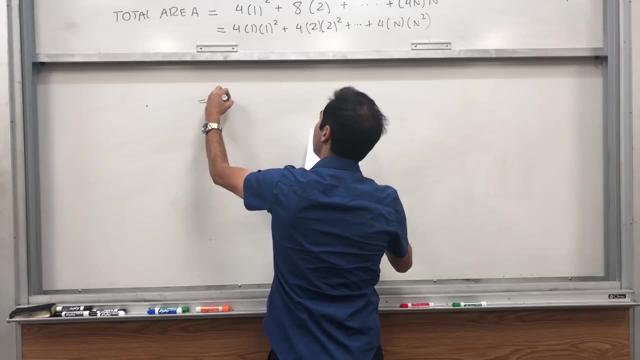 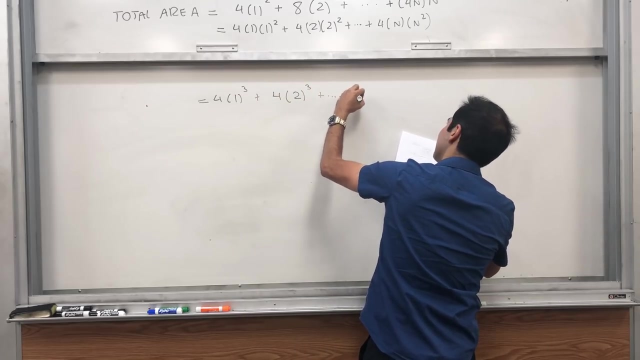 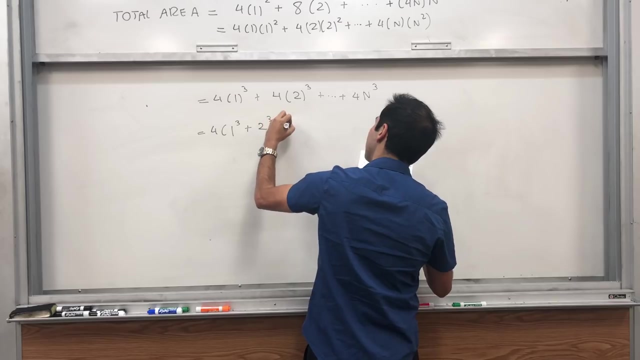 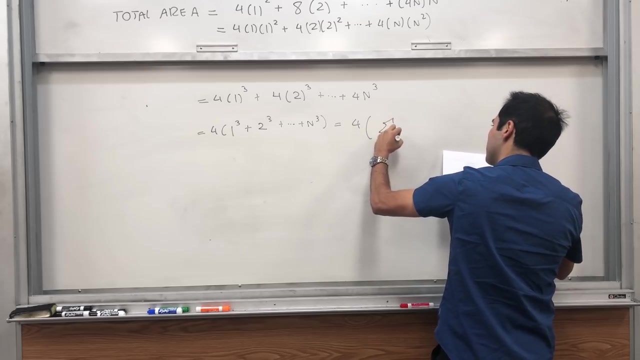 precisely 4 times 1 cube plus 4 times 2 cube, etc. etc. plus 4 times n cubed and game cube, which is precisely 4 times 1 cube plus 2 cube plus n cube, and that is precisely 4 times the sum over Qs. 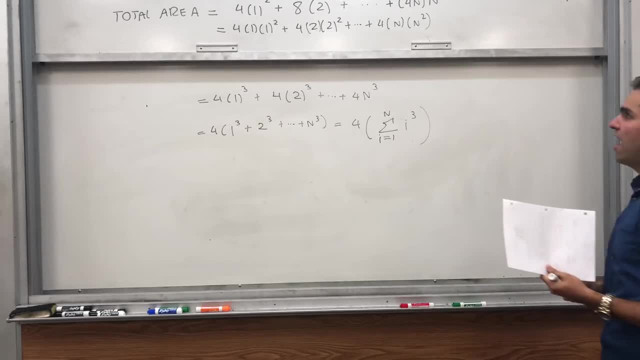 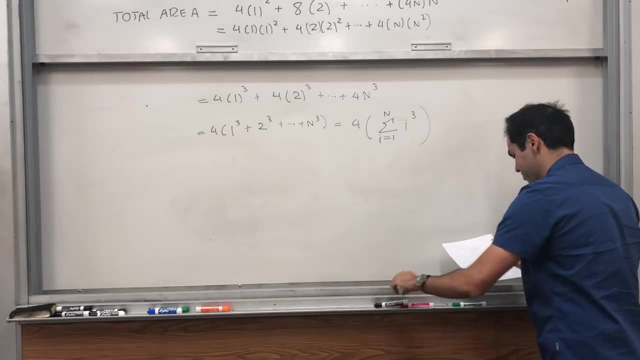 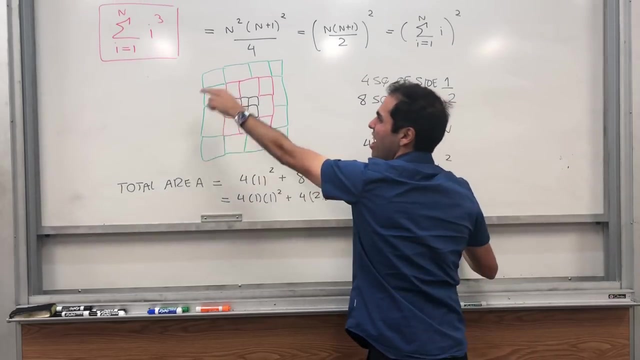 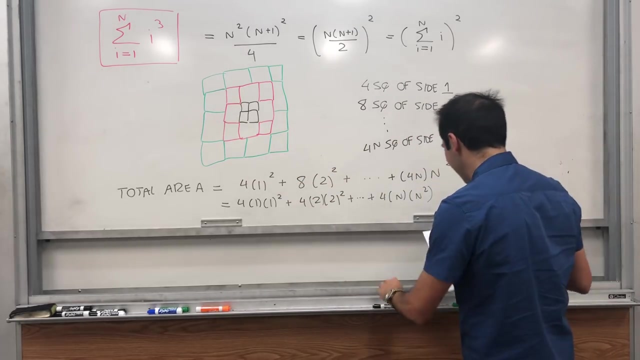 so that is one way of calculating the total area. just sum up the areas of this square. on the other hand, in this is the cool thing- this geometric figure is itself a square, so you just have to calculate the total side length and square it and notice what makes this. 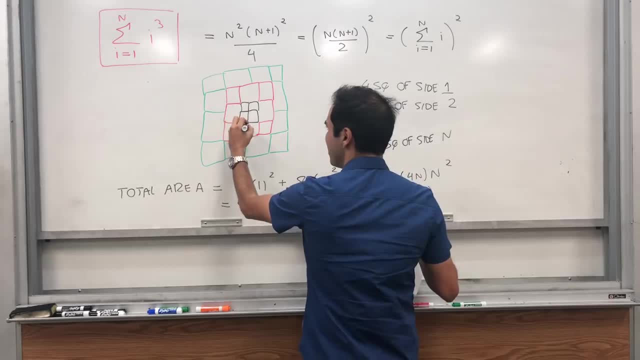 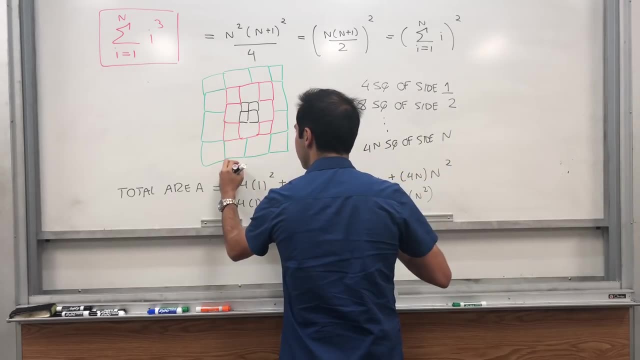 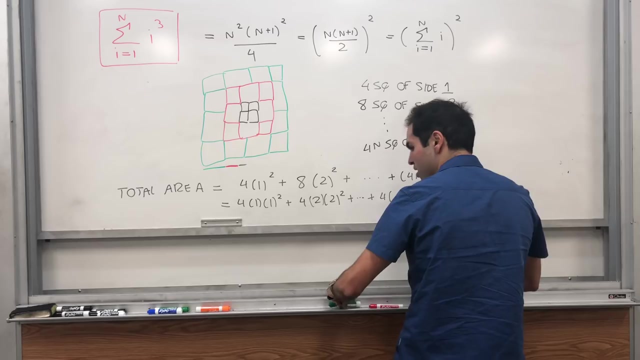 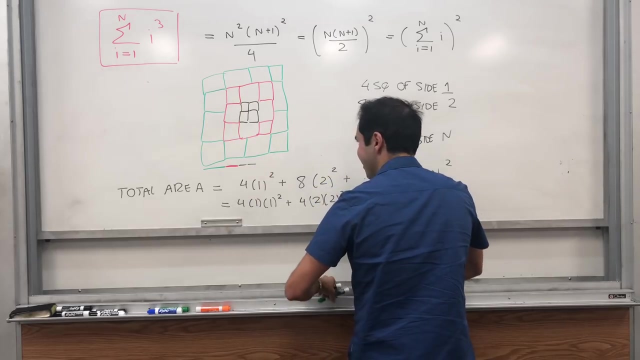 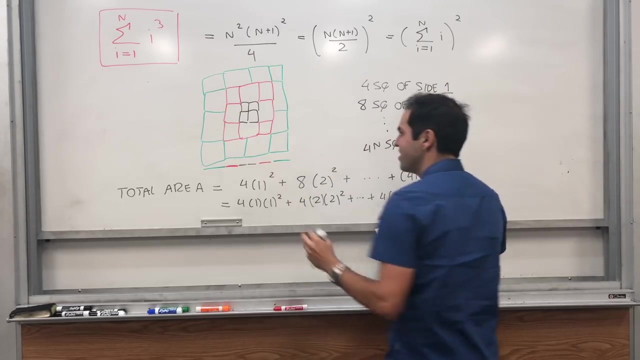 nice, there's this projection thing going on, because if you project it on the axis, you get the small square, then the medium square and then the big square, and you double-count it. so we have this pen, this black pen, red pen today, so, and green pen. so you see what is the side of the big square? it's precisely one plus. 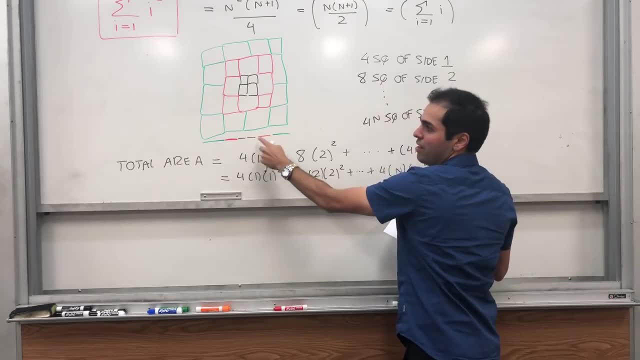 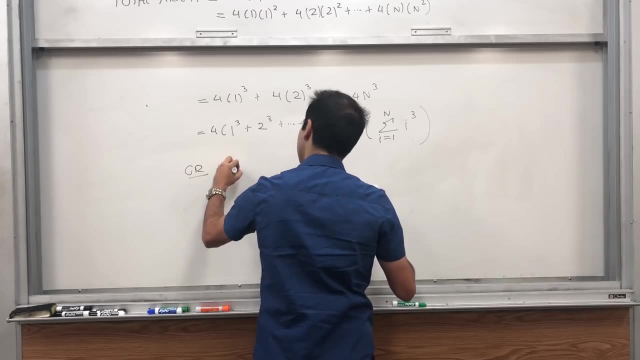 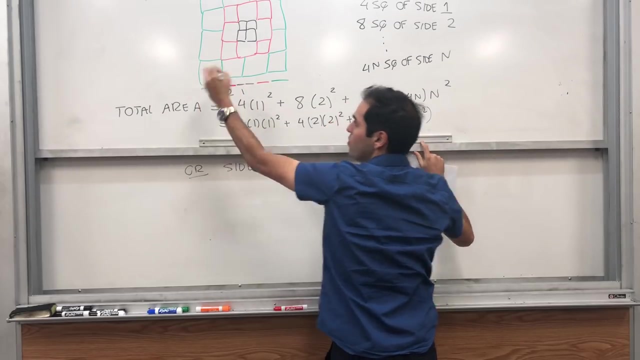 two plus three and plus one plus two plus three, so it's the gradation of the square, and so forget what else you saying. you can- I really double that- so or you can say the side is again 1 plus 2 plus 3 and we. 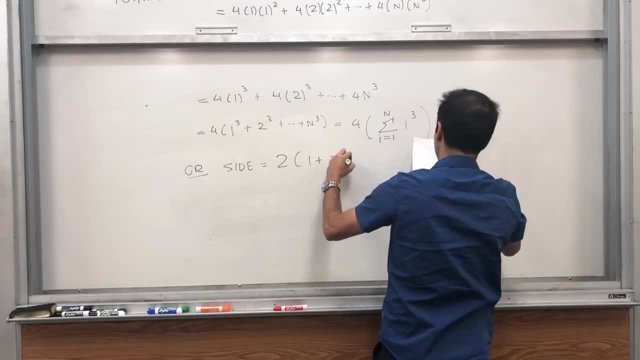 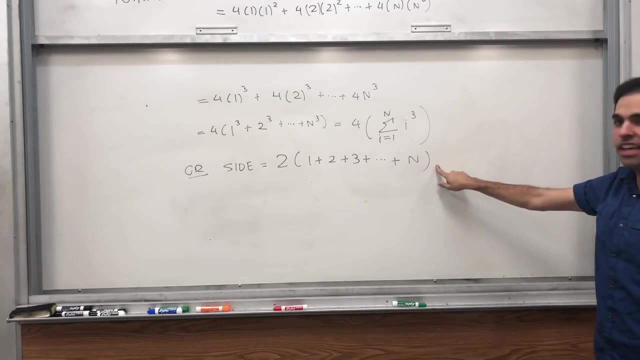 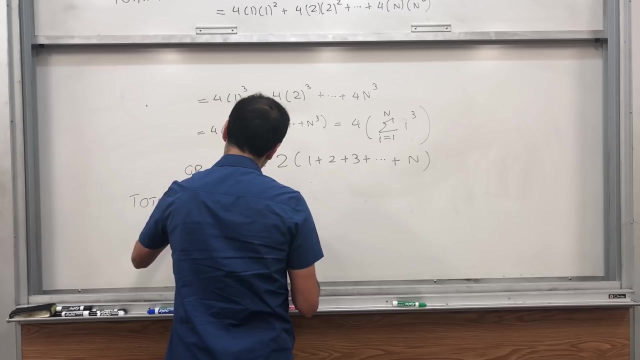 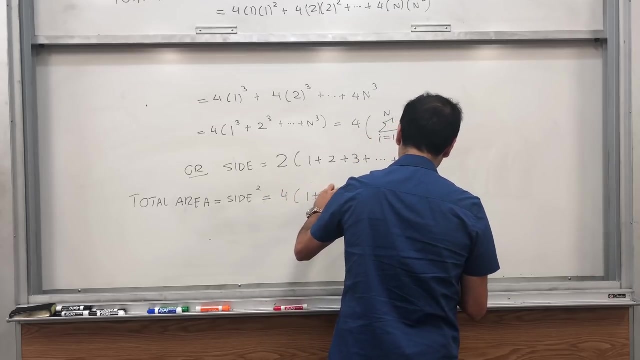 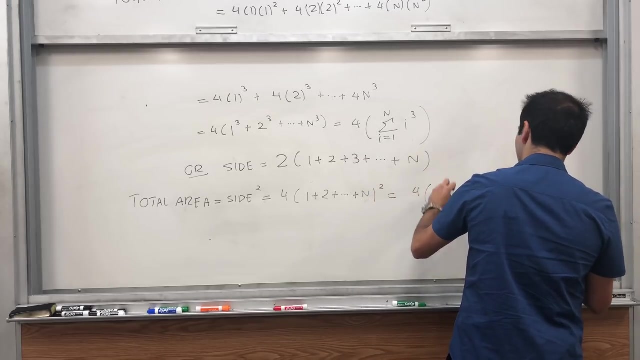 double that, so 2 times 1 plus 2 plus 3, up to n. so what is the total area? is the side squared? total area is side squared. and that then just becomes 4 times 1 plus 2 plus dot, dot, dot plus n squared, which is 4 times the sum of the integers. 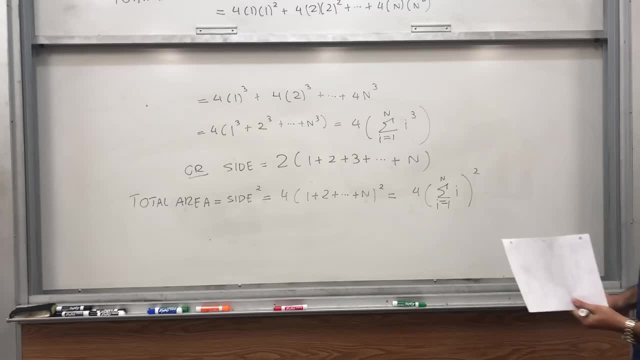 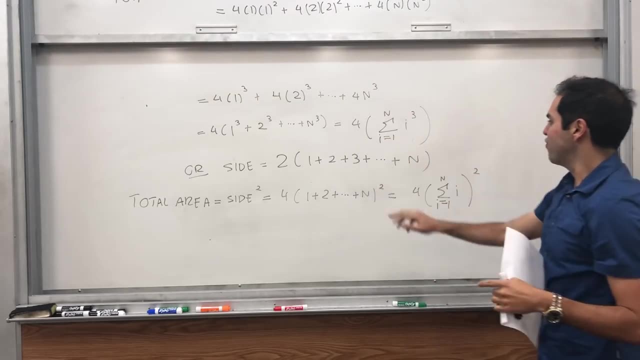 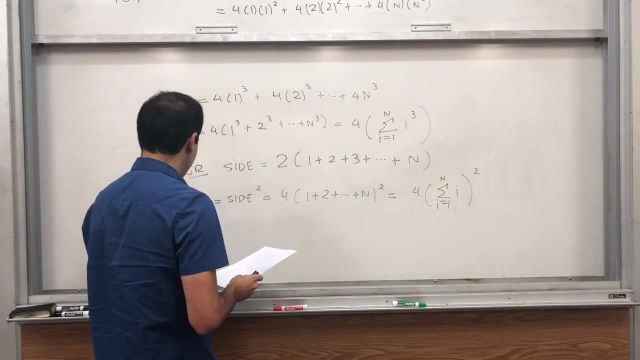 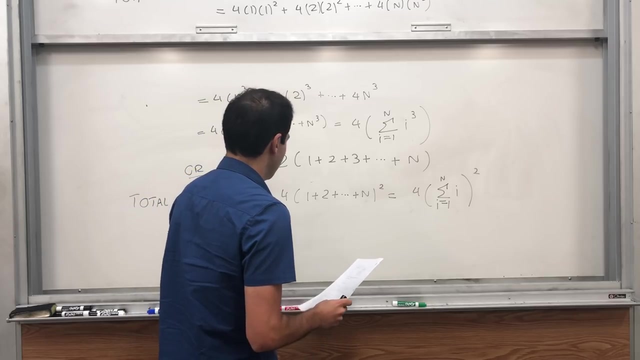 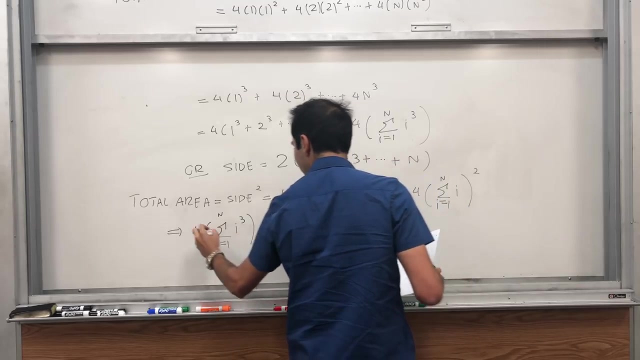 squared and therefore, because both quantities are calculated in the same area, what we get is that four times this quantity equals four times this quantity. in other words, exactly what we want. four times the sum of cubes- i cube- equals 4 times the sum of the integers squared. you cancel out the 4 and.